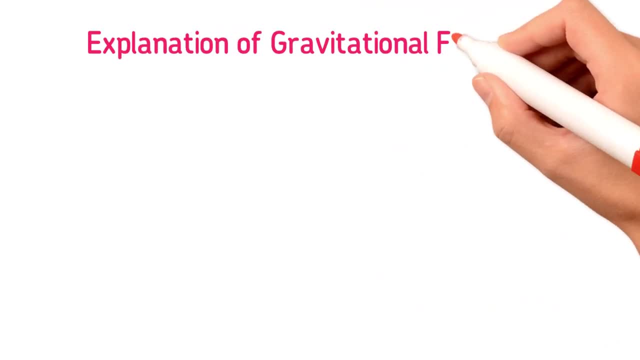 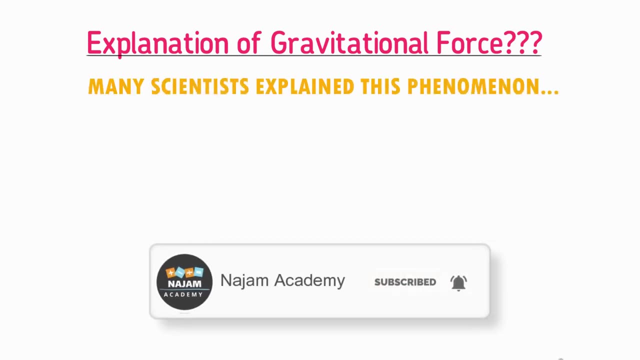 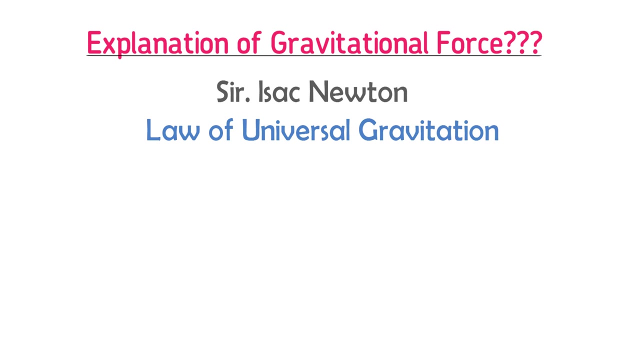 Now the first question is that: who explained the gravitational force in physics? The answer is that many scientists explained the phenomena of gravitational force, But Sir Isaac Newton is among the prominent scientists who presented his famous law of universal gravitation. According to this law, we can calculate gravitational force between any two masses, either the two. 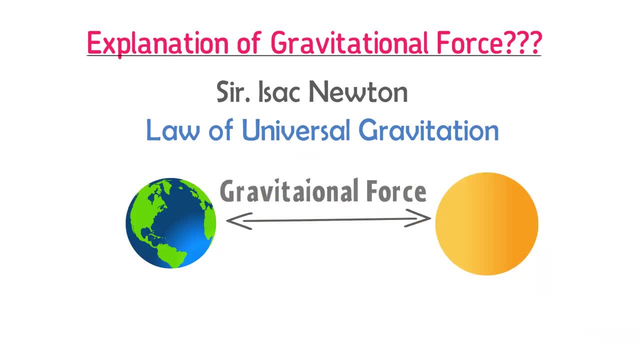 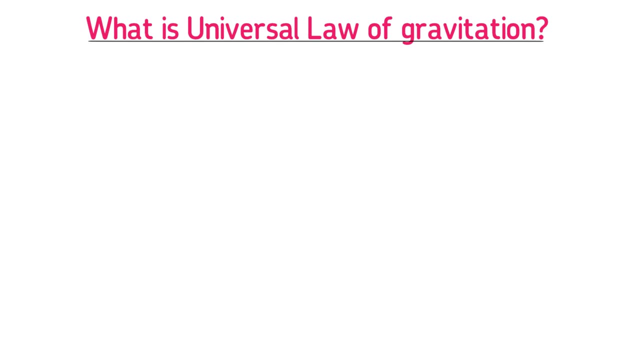 masses are living bodies or non-living bodies. Now, what is universal law of gravitation? Universal law of gravitation states that there will be a gravitational force between any two masses or any two bodies. For example, let consider that we have two bodies or two objects. 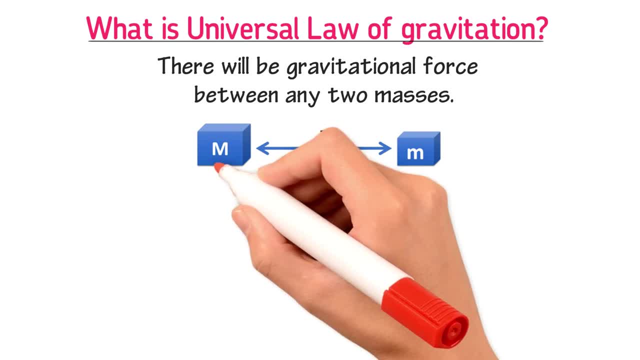 Let the mass of this object is M and the mass of this object is M. Let the distance between the center of this object is M. Let the distance between the center of this object and this two object is R. Now, according to Newton's universal law of gravitation, there is a gravitational 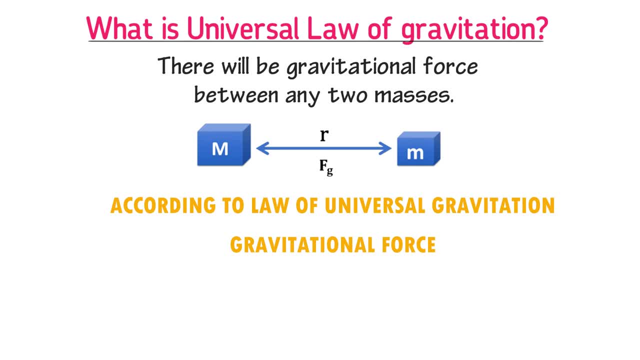 force between these two masses, Or you can say that there is attractive force between these two masses. Let we call this attractive force or gravitational force as Fg. Now, if someone asks Newton that how much gravitational force or attractive force, Fg, exists between these two masses, Newton answers this question as the gravitational force Fg depends upon. 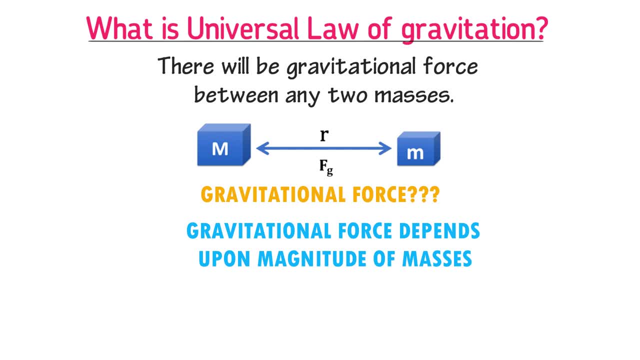 the magnitude or size of these two masses. Newton states that Fg is directly proportional to the product of magnitude of mass. Now, the gravitational force Fg is the ratio of capital M and small m. Let I call this equation number one. Secondly, Newton states that gravitational force Fg is inversely proportional. 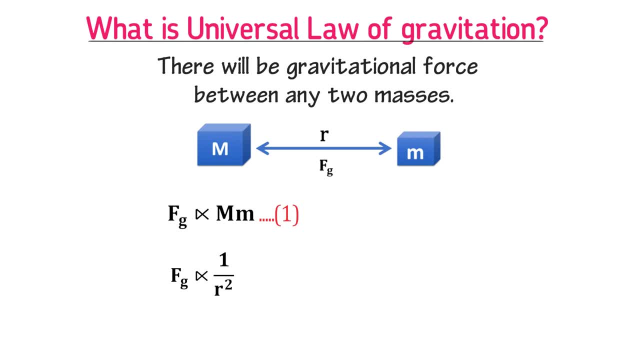 to the square of distance between these two masses. Let I call this equation number two. Now, combining equation number one and equation number two, we get Fg is directly proportional proportional to the product of magnitude of masses and inversely proportional to the square of distance between the center of masses. 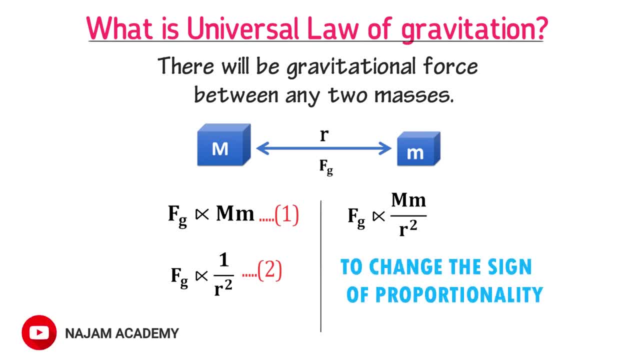 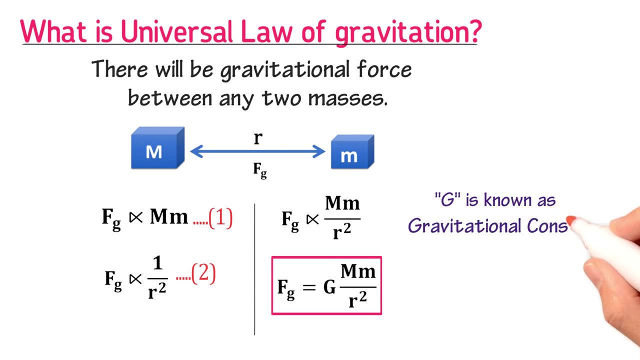 Now to change the sign of proportionality we need to put a constant. Thus Fg is equal to G Mn2m divided by R square. Here the G is known as a gravitational constant and its value is equal to 6.67 x 10 to the. 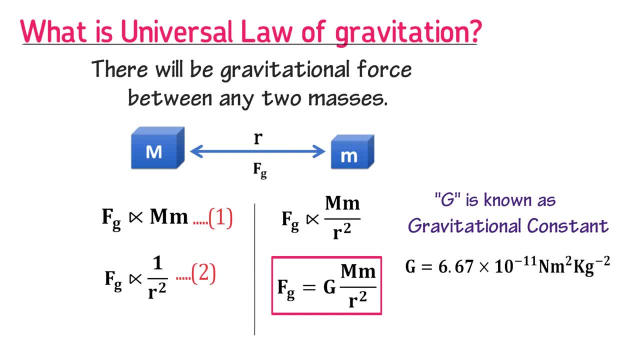 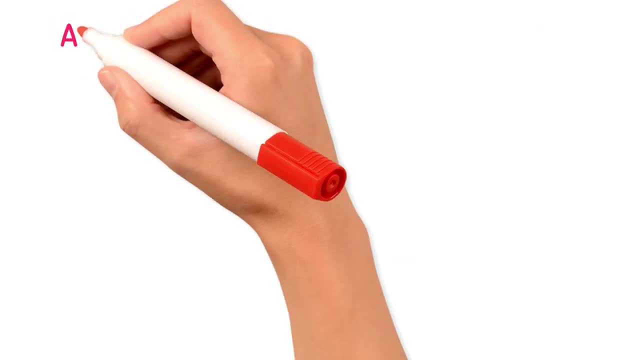 rise power minus 11 Newton meter square per kg square. Thus this law is known as a universal law of gravitation, which gives us the gravitational force between any two masses. Here remember that according to the normal law of gravitation, the gravitation of mass 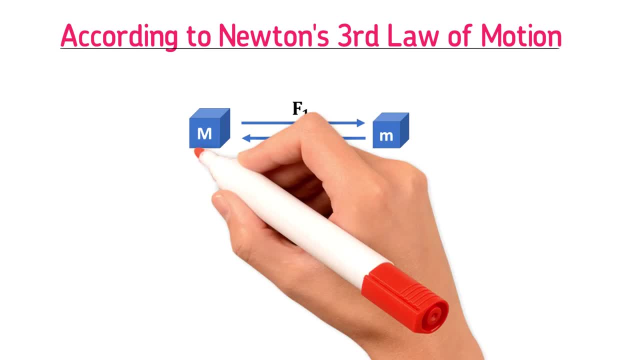 and mass is proportional to the force between any two masses. Here remember that according to normal law of gravitation, the gravitation is proportional- Newton's third law of motion. if this mass m exerts force F1 on this mass m, then this: 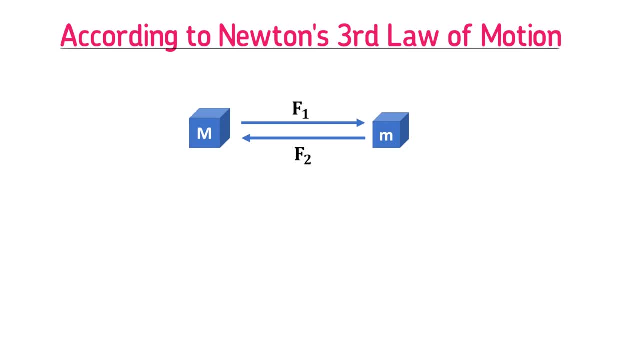 mass or this object also exerts force F2 on this mass or this object. For example, if the earth pulls on the moon, the moon also pulls on the earth with a force of equal magnitude. You can understand this example as if 1 kg body is present above the earth's surface. 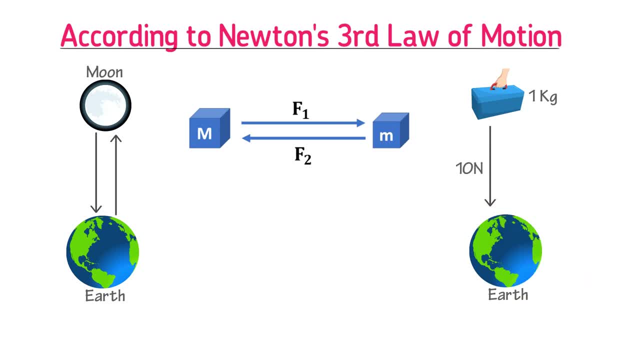 The earth exerts roundabout 10 N force on this 1 kg object, while at the same time this 1 kg object also exerts 10 N force on the earth. The mass of the earth is larger than the mass of this 1 kg object. 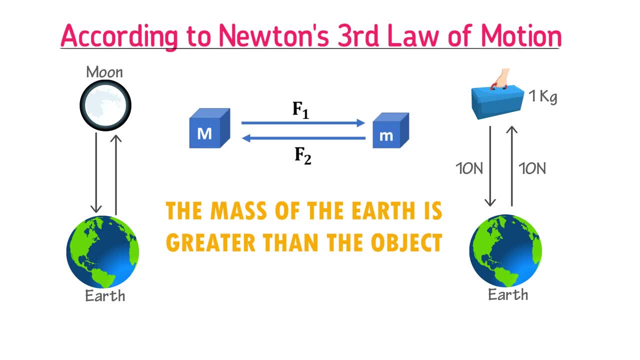 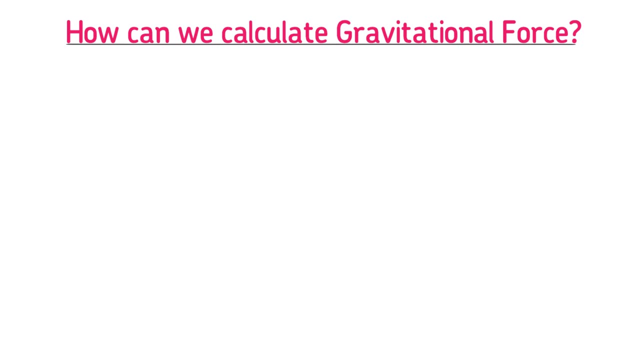 That's why the earth is so large. The earth doesn't accelerate towards the object, but the object accelerates towards the earth. Now, at last, let me teach you that. how can we calculate gravitational force between any two masses or objects? Let's consider that a boy is standing here and a girl is standing there. 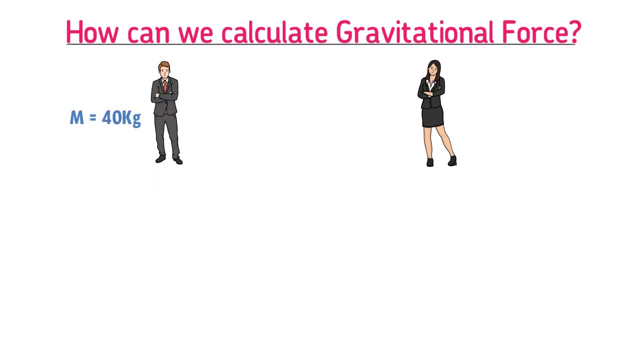 Let the mass of the boy, capital M, is equal to 40 kg And the mass of the girl, small m, is equal to 45 kg. Let the distance between the boy and the girl R is equal to 0.5 meter And the gravitational force between the boy and the girl is Fg. 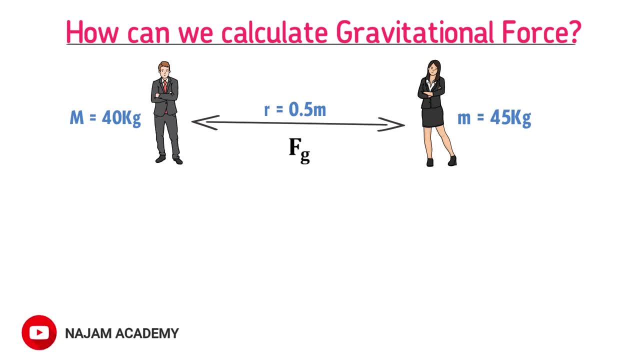 In order to find the gravitational force between the boy and the girl, we have to use the Newton's law of universal gravitation, Which is Fg. Fg is equal to g, m into m divided by r square. Here, capital M is the mass of the boy. 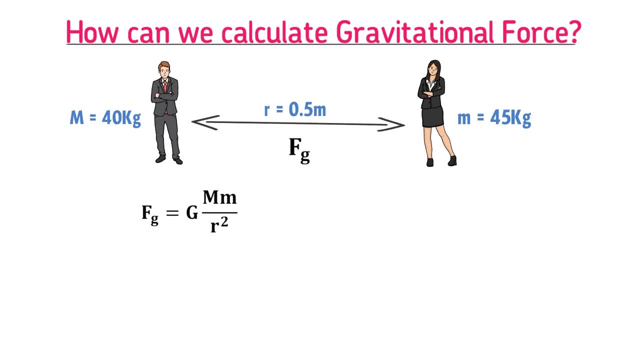 and the smaller, m is the mass of the girl and r is the distance between the boy and the girl, While we know that g is the gravitational constant and its value is equal to 6.67 into 10, to the rise power minus 11.. 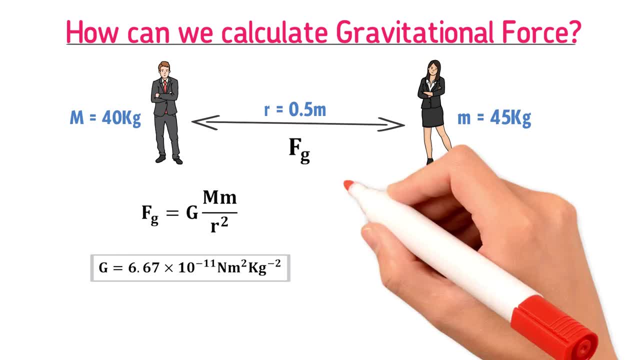 Thus we will put the values in the formula: Fg is equal to 6.67 into 10, to the rise, power minus 11 into 40 into 45, divided by 0.5 whole square, Hence, Fg is equal to 6.67 into the power minus 11. 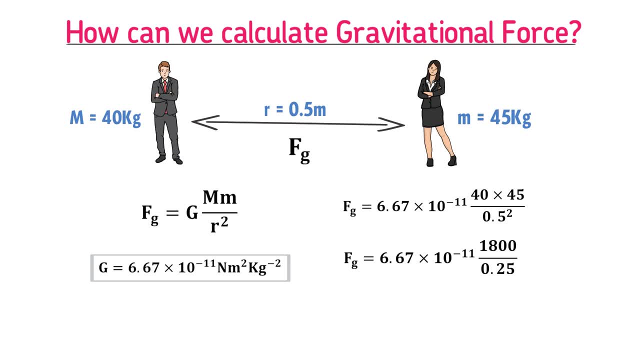 multiplied with 1800 divided by 0.25.. Or we get: Fg is equal to 6.67 into 10 to the rise power minus 11. Fg is equal to 4.8 into 10 to the rise power minus 7 newton. 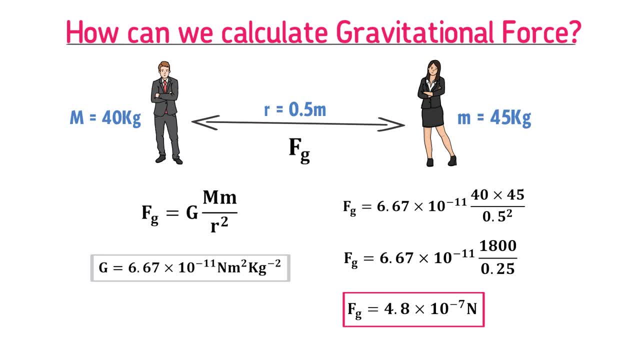 Thus the gravitational force between the girl and the boy is about 4.8 into 10 to the rise power minus 7 newton, which is extremely small force. That's why the boy and the girl do not feel the gravitational force between them. 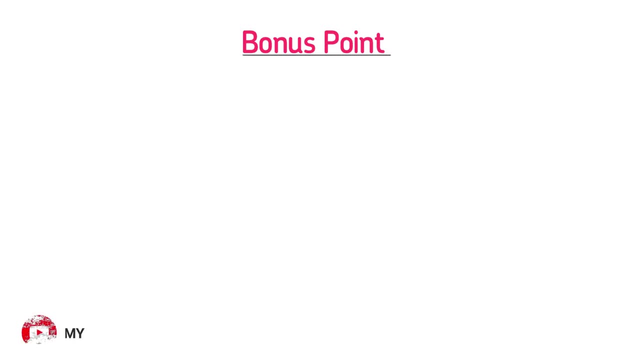 At last. let me teach you one bonus, As we know that gravitational force is directly proportional to the product of masses And gravitational force is inversely proportional to the square of distance between the centers of two objects. If the distance increases two times between any two masses, the gravitational force decreases. 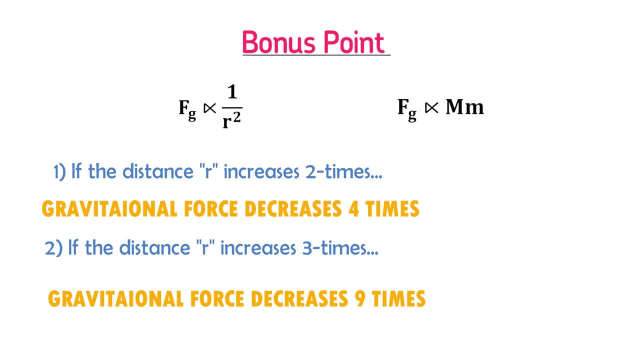 four times. If the distance increases three times between any two masses, the gravitational force decreases nine times. If the distance increases 15 times between any two masses, the gravitational force decreases nine times. Therefore, we say that gravitational force follows the Inverse Square law.